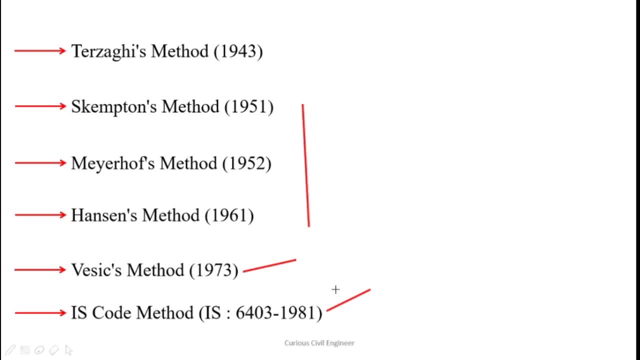 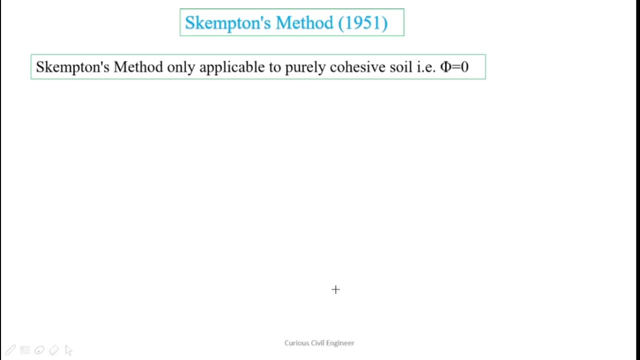 And having a little bit of knowledge more than what is required never hurts you. Okay, So please follow the entire video. We will start with Skempton's method 1951.. So the Skempton method is only applicable to the purely cohesive soil, So a clay soil, which 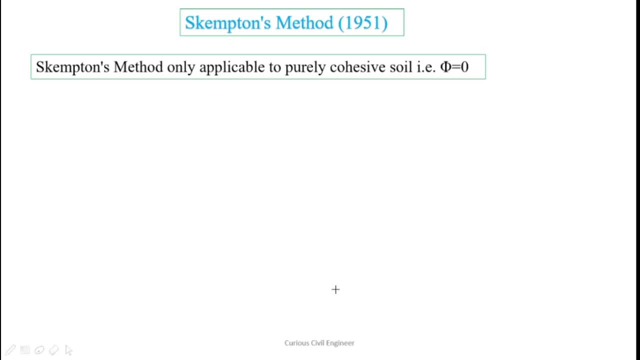 has phi equals to zero. This Skempton's method is applicable to that. Okay, So Skempton method, ultimate net, ultimate bearing capacity, is given by a very short formula, That is: q net, ultimate equals to c, n, c. It's a very short and sweet formula. Other thing about this Skempton's method is: 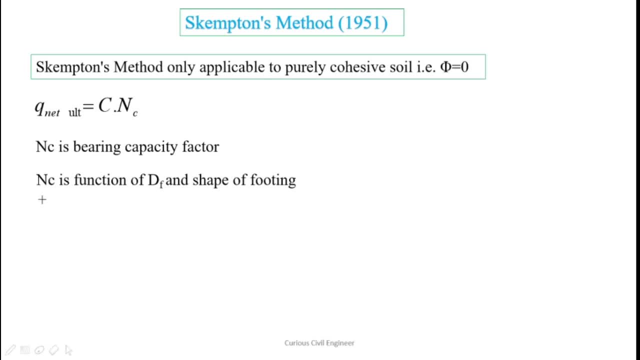 that the value n c does not depend upon the value of phi, Because in Terzaghi's method we had seen n c, n, q, n, gamma. It depends upon the value of phi, But here n c depends upon the value of d, f and the shape. 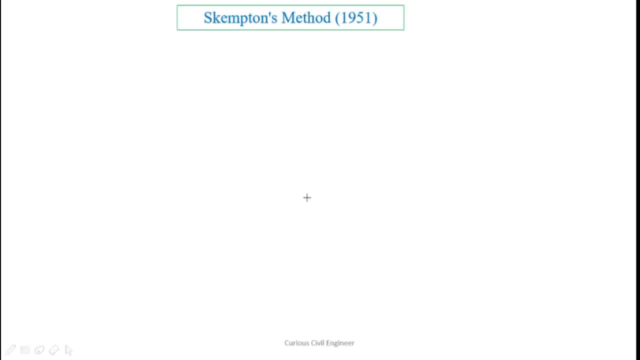 of footing. Okay, Now for the stripped footing. the value of this n c equals to this. So because for the different, as it depends upon the shape of footing, For different shape, for stripped footing or continuous shaped footing, you will have a different value of. 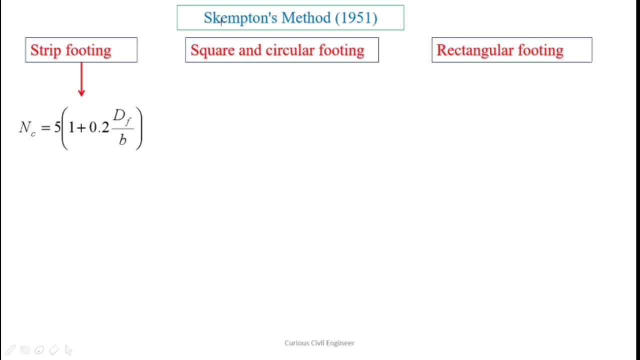 n, c. For square and circular footing, you will have a different value: n, c, n, q, n, gamma. Now for footing, you will have a different value of NC. for rectangular footing, you will have a different value of NC. so the first for strip footing. this is a. 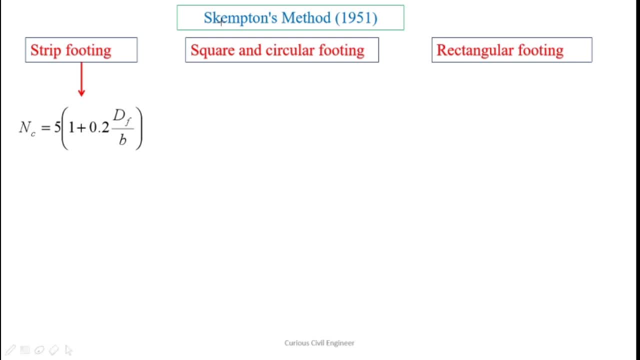 formula given over here that is used for determine NC value, and the value of NC is restricted to 7.5 for value of DF by B greater than 2.5. so let's say, if the ratio of DF by B is going beyond the value of 2.5, what you will do. let's say: 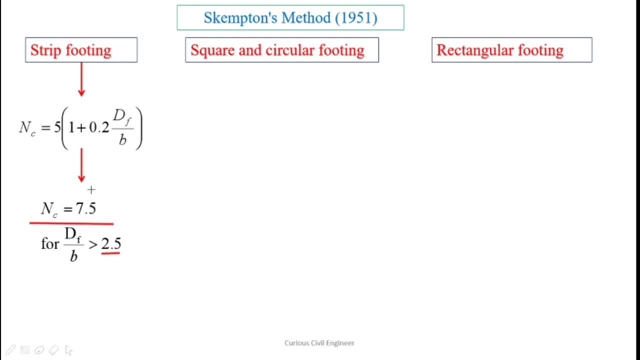 your DF by B is 3. so what you will do? just take the value of NC equals to 7.5, that's it, okay. and for the square footing you will have a different formula, which is given over here, and this value is restricted to 9, okay, so? 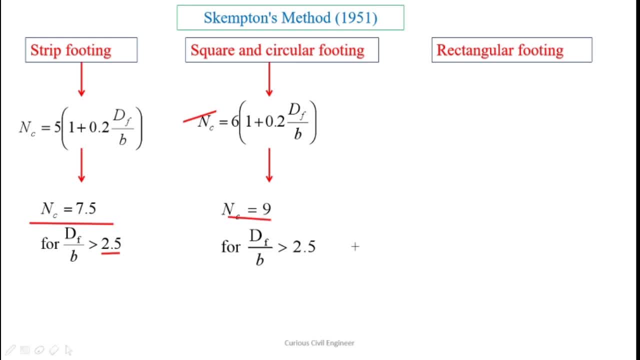 let's say your DF by B is, let's say 2.6. so let's say your DF by B is, let's say 2.6. so let's say your DF by B is, let's say 2.6. so what you will do? just take the value of NC as a 9. that's it for rectangular. 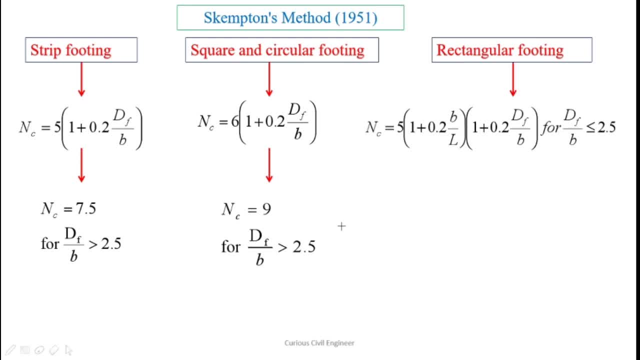 footing. the formula is lot more complex and this formula is this: NC equals to this big formula over here. L is the length of the footing, B is the width of the footing, DF is the depth of footing from the ground level. okay, and this formula is applicable for DF by B. 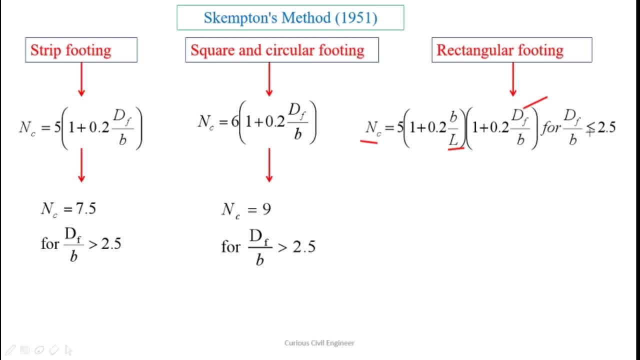 less than 2.5, less than equals to 2.5. if this DF by B goes beyond the ratio 2.5, then you will have to use this formula. okay, and one of the good thing about this Kempton's method, why it is still relevant even though we have different. 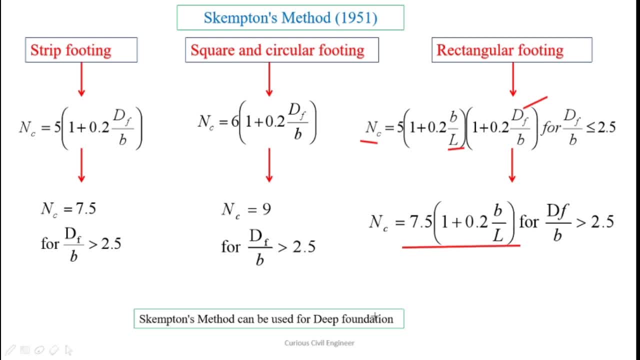 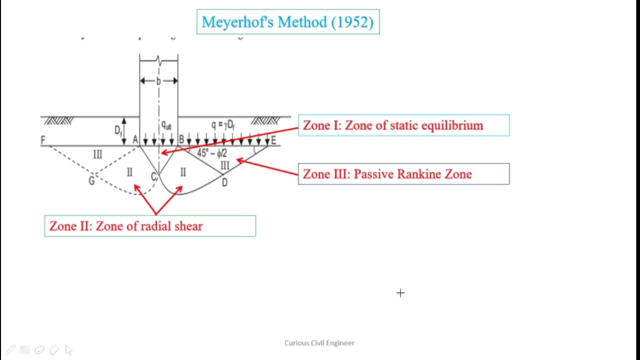 methods, because this method is applicable to deep foundation also- remember Terzaghi's formulas- or not applicable to the deep foundation directly, but you can use Skempton's formula for deep foundation also. that's why it is still relevant after so many years. next one: Mierhof's method, 1952. now on the screen, what you see over here is this is the. 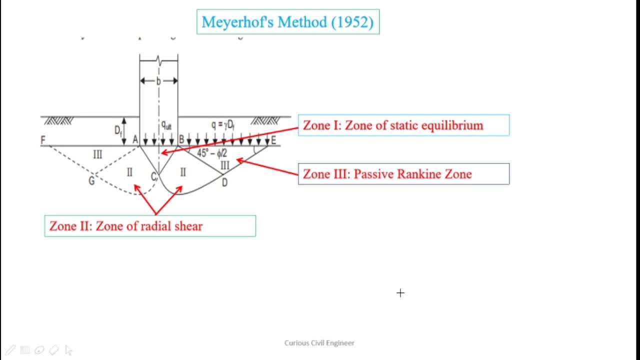 zone in which the Terzaghi has divided the soil below the base of the footing. so we- I think we have seen this in part 1 of the shallow foundation series- zone 1, zone 2, zone 3- and one of the basic assumption of the Terzaghi was that all 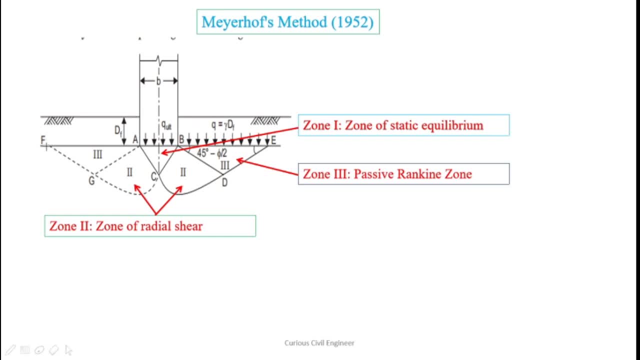 these three zones are below the base of the footing. so if this level that I have shown you over here, Fe, is the zone of the sorry base of the footing, then these three zone will always remain and the base of the footing will always remain below the base of the footing. but Mierhof says that these zones may exceed. 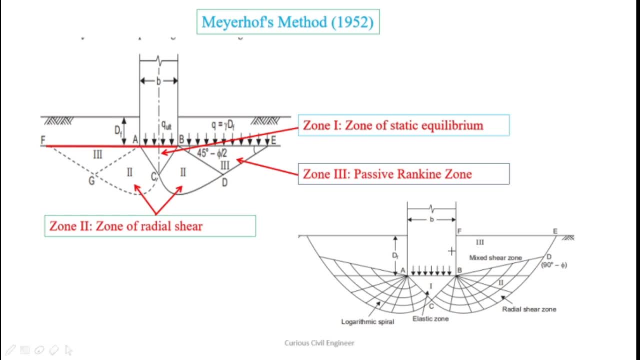 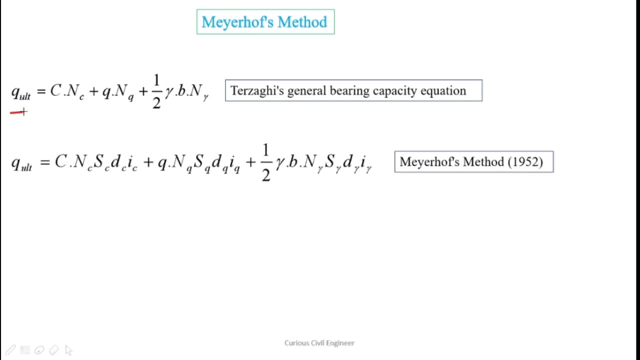 beyond the base of the footing. so he has given additional zone that is called a mixed shear zone. okay, and this is your Terzaghi's formula, which is given over here, and the Mierhof's formula is lot more bigger than Terzaghi's formula. okay, 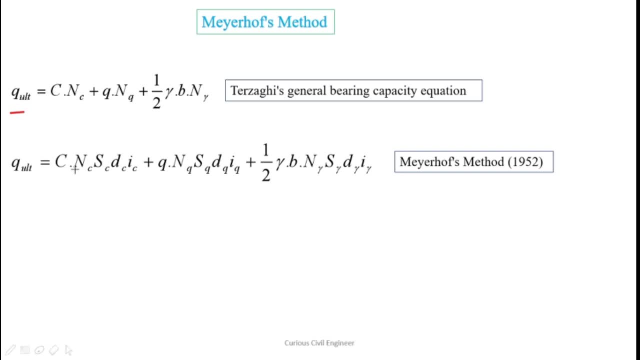 and what are these values that you see over here? SC, DC, IC. these are called as a this, SC, SQ, S, gamma are called as a shape factors. DC, DQ, D, gamma are called as a depth factor. IC, IQ, I, gamma are called as a inclination factor. okay, next Mierhof. 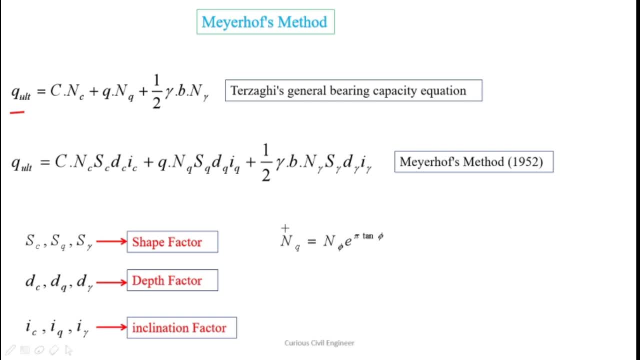 has also given different value of NC, NQ and gamma. so for the nq you have to use this formula in merov and this value, nphi, in this formula of nq, is nothing but tan square 45 plus phi by 2. next is the value of nc, that is equal to nq-1 cot phi. 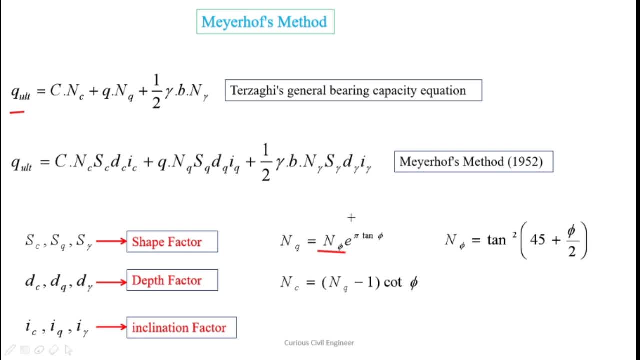 now, other important thing that you should remember, whether it is a merov method, hansen method, iscord method, wesiks method, these nq, nc and nphi never changes. these values remain constant in all the methods and value of n gamma will keep on changing, depending. 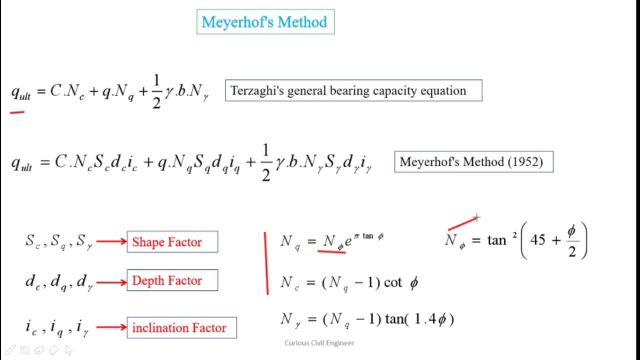 upon the different method that you are using. for example, for the merov method, the value of nq n gamma equals to nq-1 tan of 1.4 times of phi. ok, and you don't really need to remember this formula because most of the time this value 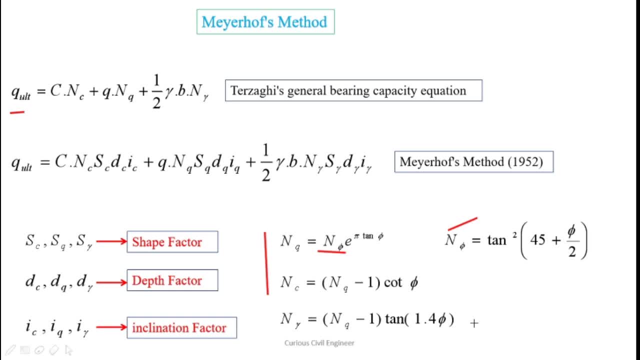 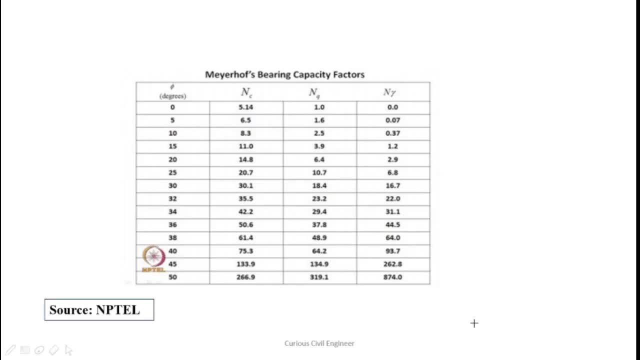 of NC, NQ and gamma are given into the numerical. if they are not given, you can either use this formula or, depending upon the method, you can also use this table. so this is one of the table for Meyerhof's. this value of NC and NQ will remain same for Wessex method. for 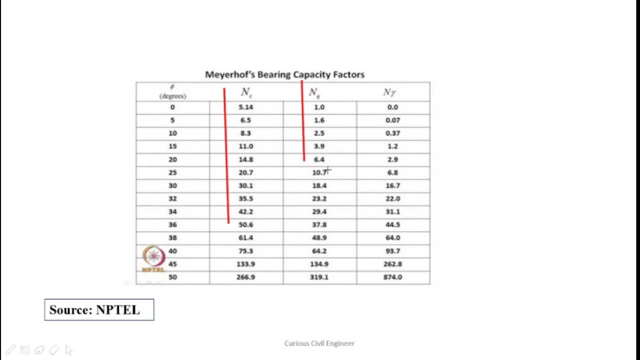 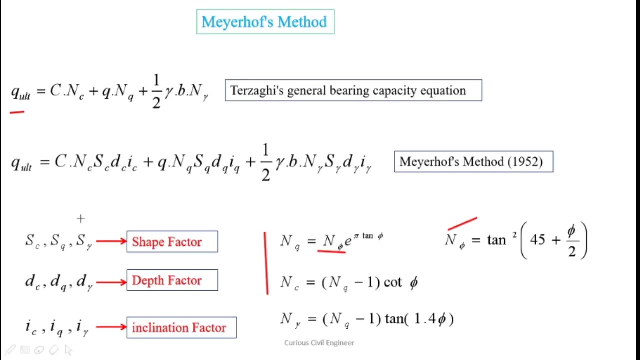 Hansen method or IS code method. the only thing that will keep on changing is the value of N gamma, because we have different formula for N gamma in different methods. ok, next, because what we have seen so far is now next thing. what we will do. we will find out the what. 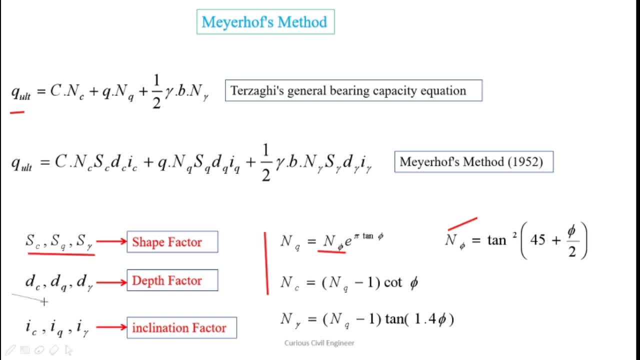 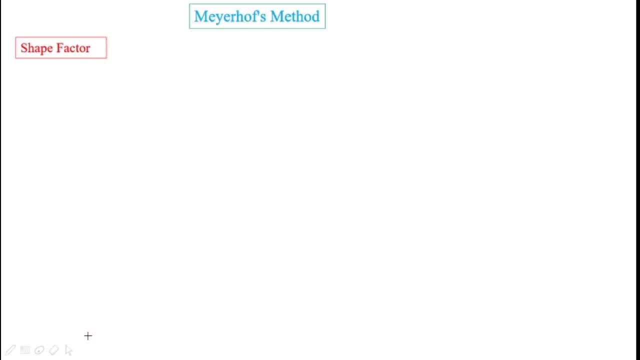 are the formulas for this shape factor: depth factor and inclination factors. ok, so let's see the first one: shape factor, shape factor. now there is a not much to explain in this. only thing that I will do is I will just show you the formula and do the whatever little explanation is required somewhere, ok, 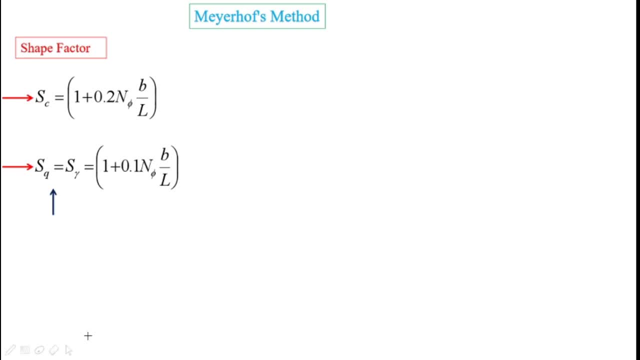 so I'm just going to show you the formula. this are the formula for shape factor in Meyerhof's method. other important thing: this formula for SQ and S-gamma is only applicable when your phi is greater than 10. if your phi is zero, SQ, S-gamma is equal to one. this is 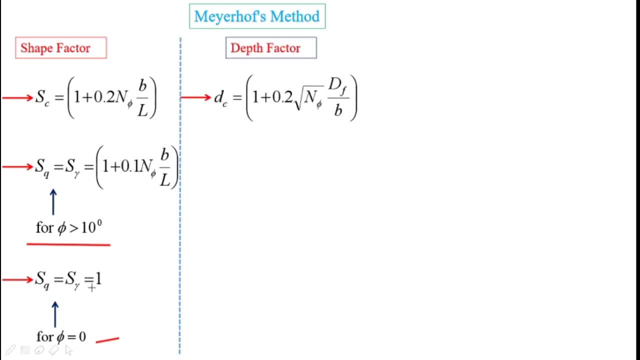 shape factor. these are the sorted方法 formulas for depth factors. ok, again, different formula for dq d gamma for different value of phi. if your phi is greater than 10, you have to use this formula. if your phi is equals to 0, dq d gamma becomes 1. so there is not much to explain, so i will just keep on scrolling. 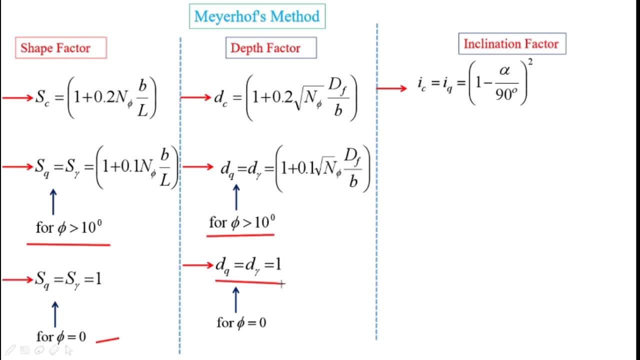 here inclination factor. this one is little bit complex so we will do some explanation over here. ok, so the inclination factor i c equals to i q and equals to 1-α by 90 degree whole square. now the important thing that you should remember: in wether it is i 240. 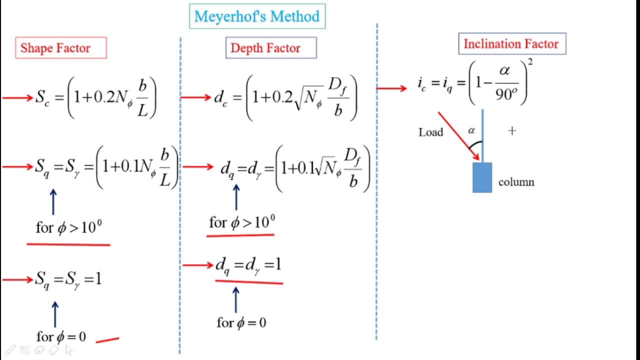 method, v6 method or any method, this value of alpha is always measured with the vertical. ok, so let say, in numerical, it is given that the load is inclined at an angle 80 degree to horizontal. ok, for that case, if we put this value of alpha at angle 80 degree to horizontal, we Height. 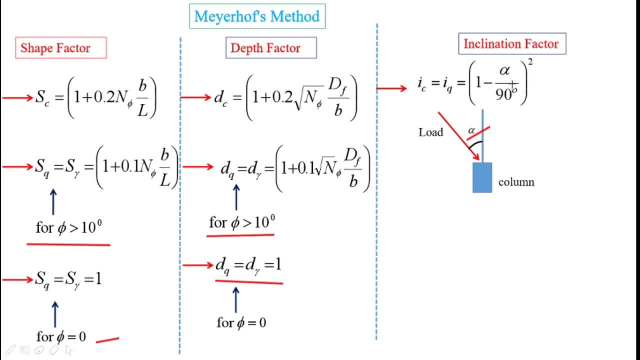 factor like this in love means the value of alpha is always measured, means that the value of alpha is always measured for angle, squared average of the numeric value and and angle at alpha that you will put over here will not be 80 degree, it will be 90 minus 80 degree, that is 10. 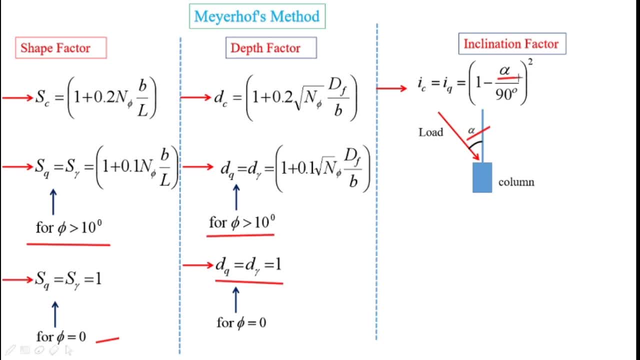 degree because alpha is always inclined with the vertical. that is very crucial, should remember. many people makes mistake over here. don't make silly mistakes here. okay, that is the value of ic and iq and this is a formula, for i gamma this straightforward. you need to remember the formulas. 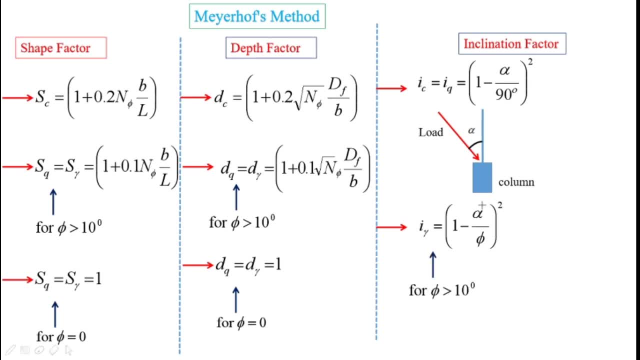 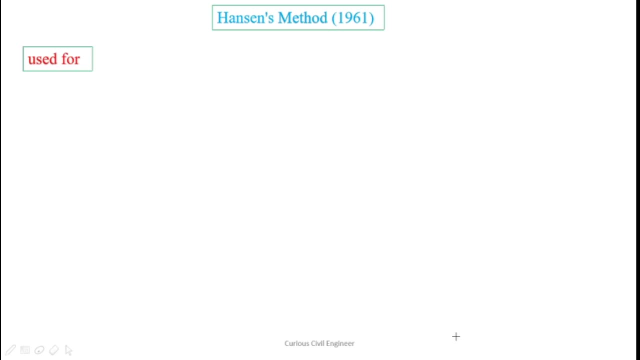 okay, and this formula is applicable if your phi is greater than 10. if your phi is 0, your i gamma becomes 0. so this is all about mayerhoff's method. next we will see the hansen method. hansen method: it is important because this method is basically used in three different condition. because 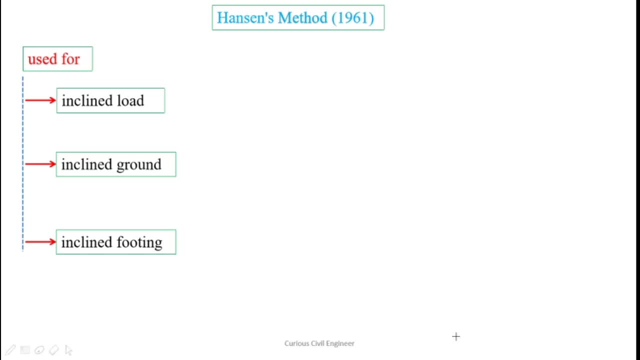 terzaghi's method cannot be used when your load is inclined. terzaghi's method cannot be used when your ground is inclined. same it cannot be used when your load is inclined. so this is all about use when your footing is inclined. so in these cases, in practical application, you need either: 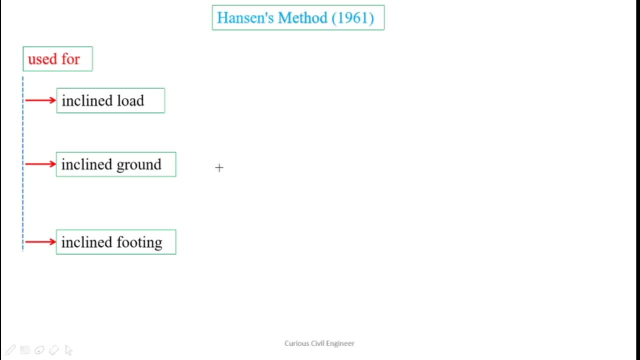 hansen's method, basics method or hascode method. okay, so hansen's formula is same as mayerhoff's formula. the only difference is the value of n gamma. if you could remember, we had a different formula for n gamma in hans mayerhoff's method. you will have a different formula for n gamma. 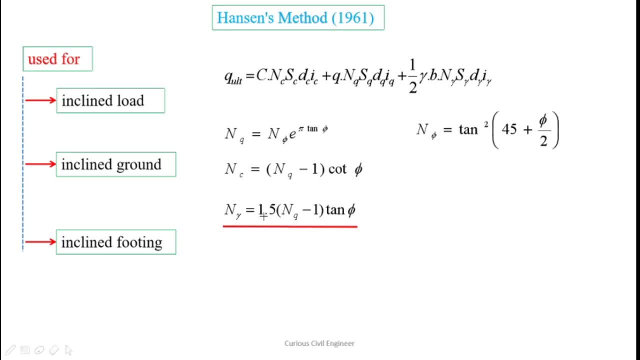 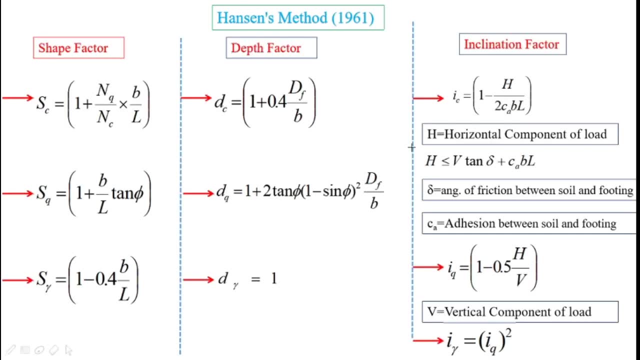 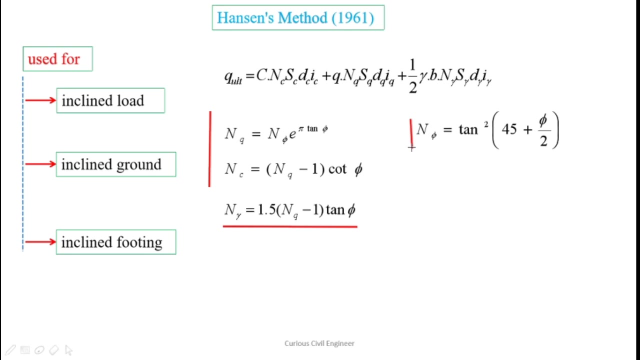 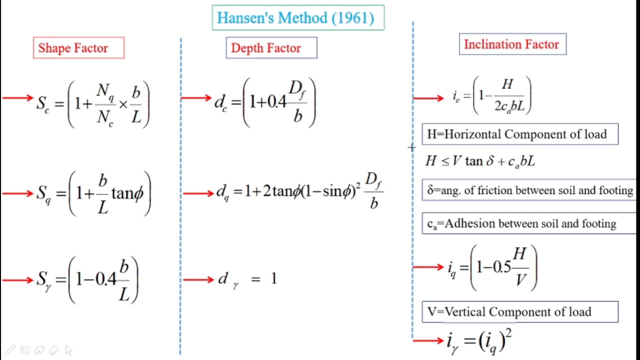 n gamma in hansen's method. okay, this nqnc is same, n phi is also same. and these are the formulas for this. shape factor, death factor, inclination factor- this is a formula given over here. i will not do an explanation over here. it is not required unless there are some critical cases like inclination factor over here. these are: 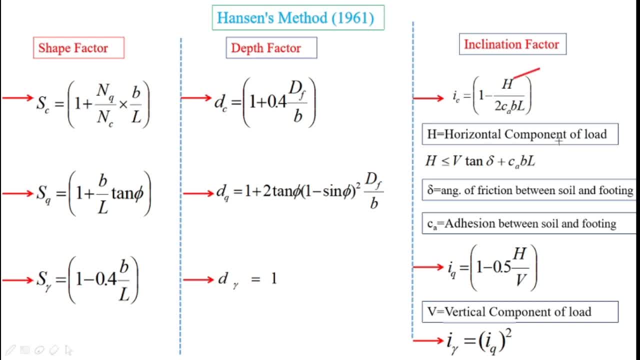 this is a different notation. h, h is nothing but horizontal component of your load is. let's say, your load is inclined, so it will have two component. one will be horizontal component, other will be the vertical component. so your h is nothing but this horizontal component and your v is: 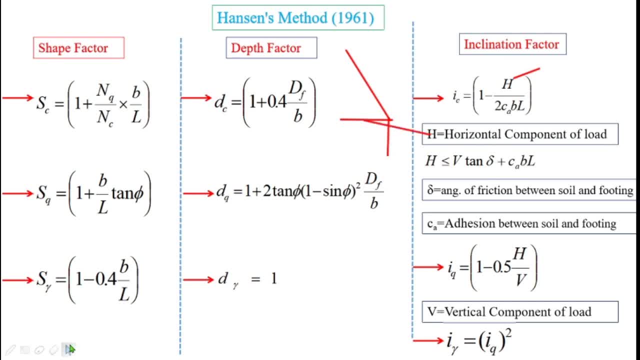 nothing but the vertical component and that's it okay. other thing is this: delta. delta is angle of friction between soil and footing. c is the addition between soil and footing. these are all if it is given into the numerical use it and it is not part of model. so it is not part of model. so it is not. 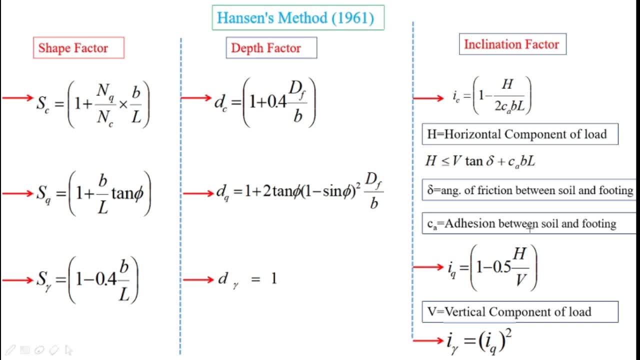 body parts. it is not part of the model. so this is the vertical component of your load. if there is vad wooden, you are given something called depth of load or Hispanics. I will try and explain why, don't any of you girls? you will not understand this process. 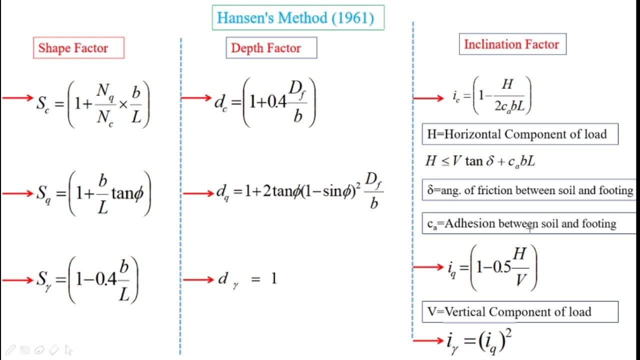 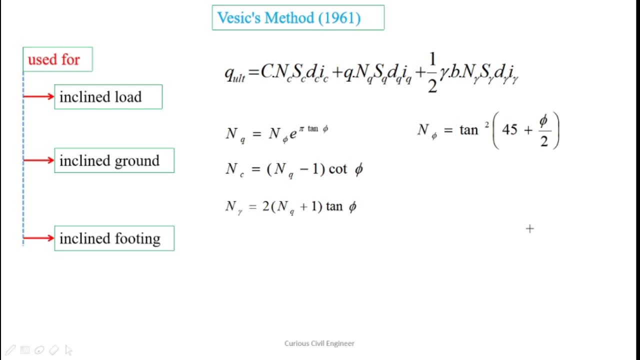 I think it is very, very important. what we are answering is this: we have to correct itself how we四 went this. okay, let's go ahead. this is important. this is part of mumbai university. you have to pay attention here over here very carefully. okay, so nqnc is same as hansen's and meerhoff no changes. 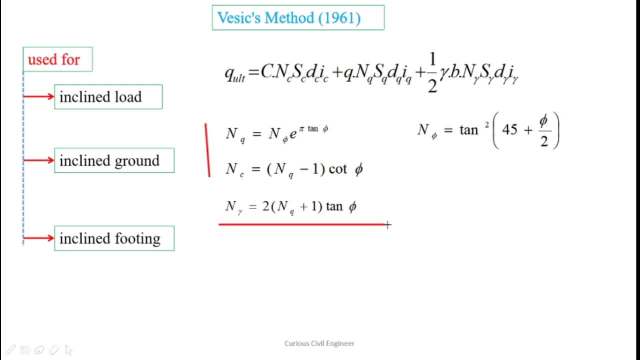 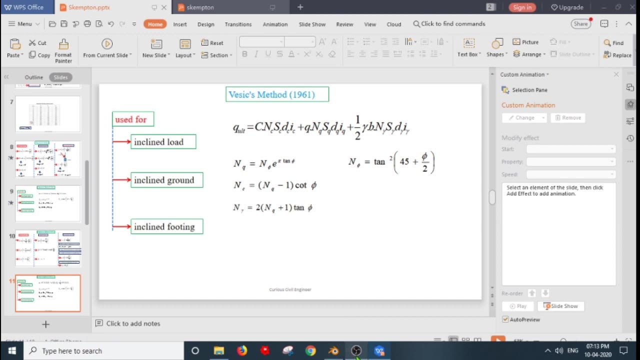 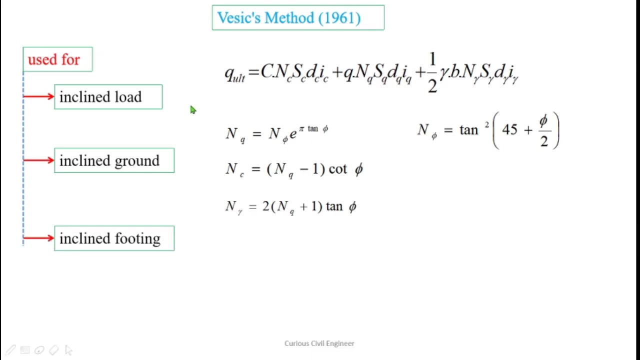 n gamma has a different formula here. you should pay attention to n gamma here, very important, okay. uh, i just forgot whether i'm recording or not, so i'll just go and check. please don't mind this. yeah, recording, thank god, okay. so basics method. you have different formula for n gamma. 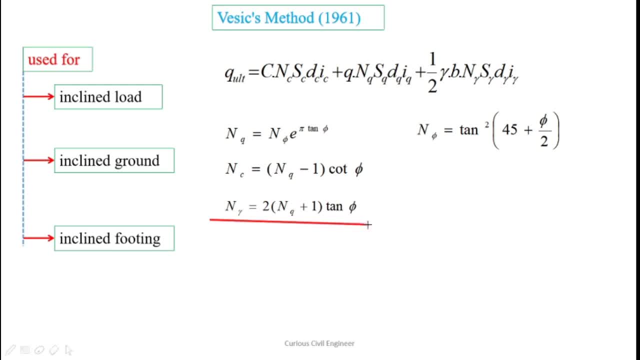 hopefully, hopefully, if you are not having a very bad luck, this value of nc, nqn, gamma will be given into your examination. if not given, please remember this formula. okay, so the only thing that we are going to see next is this shape factor, because these will not be given: sc, sq, s, gamma, dc, dq, d. 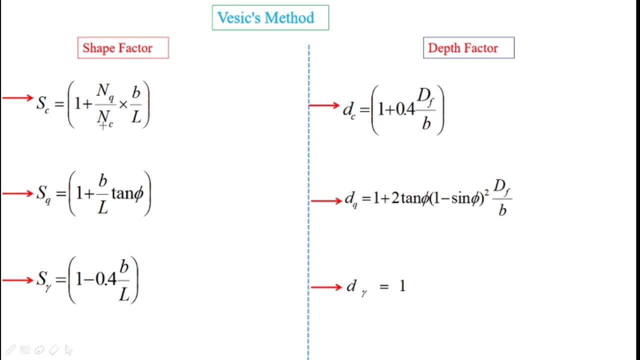 gamma, i, c, i, q, i, gamma. these values will not be given into your examination. you must remember this formula. these formulas are very straightforward. sc's formula is this and, if you can, if you could pay attention to this, these are the same formula that were used in hans hansen's method. so let's 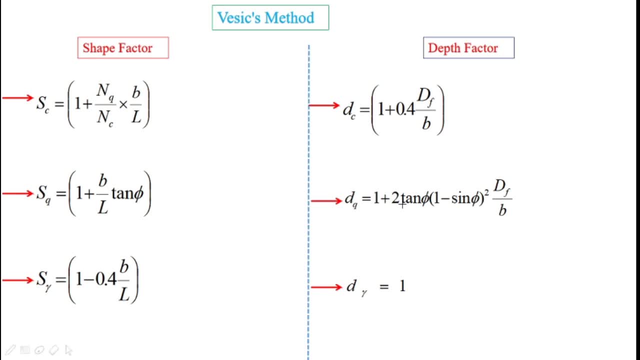 not go into the detail. these formulas are very straightforward. just remember them and use them, okay. so other important thing that we should see is inclination factor, because inclination factor needs a little bit of explanation. so the first inclination factor i see. this is a formula given and this formula is applicable for phi greater than zero. so this is usually asked in our 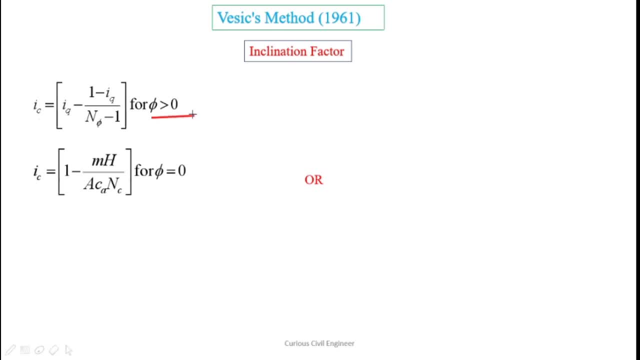 examination where phi is always greater than zero. in a very rare occasion it might happen that you have to use different formula for i c when phi is equals to zero. okay, if phi is greater than zero, your formula is very simple, very easy. if it is equals to zero, this formula where i c equals to one. 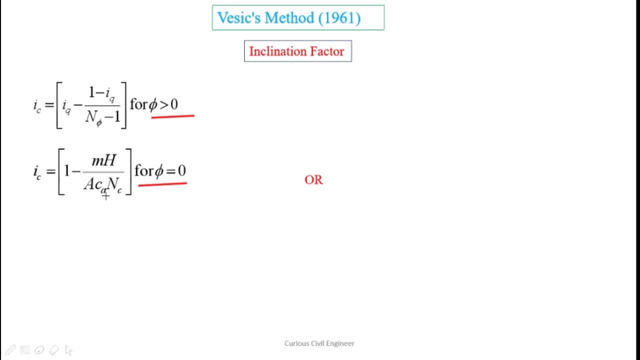 minus m by h, a, c, a, n, c, this formula, the value of m over here, is this: this is again a very big formula and there are two formulas for m to determine value of i, c when phi is zero. first formula of m is this: where b is the width of the footing, where l is the length of, 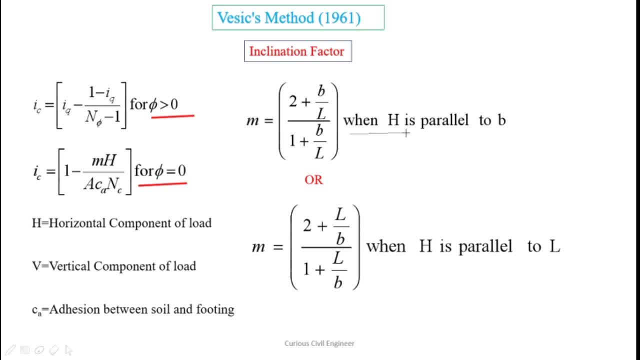 footing and it is applicable when your h- that is, remember h- is horizontal component of the load. you, if your load is inclined and it has two component: horizontal component and vertical. horizontal component is parallel to B, then in the formula of IC you will use this formula. if your H is parallel to L, then in the IC formula you will use this formula. ok, so this? 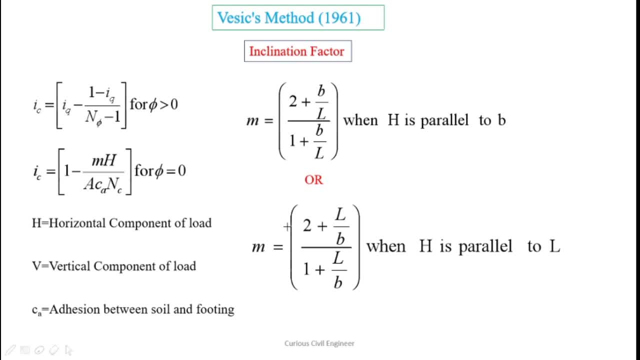 could be little bit complicated. if you don't have enough information available into the numerical and you can cannot decide, sorry. and you cannot decide whether your H is parallel to B or H is parallel to L, then don't worry, just use any of these formulas. the result: 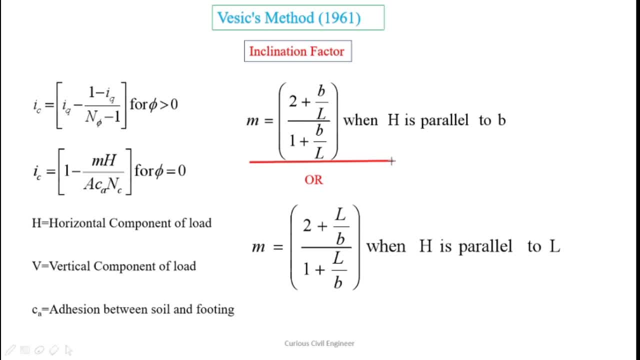 will not be like very drastically different. there will be small variation and nobody will even notice where you made mistake. ok, so just hope and pray that the value of 5, which is given to you in exam, is greater than 0. if it is not greater than 0, then you will have. 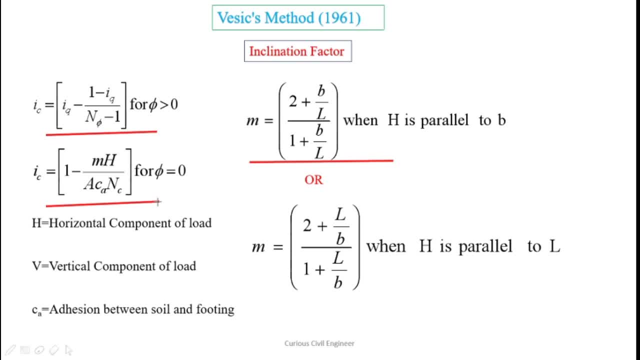 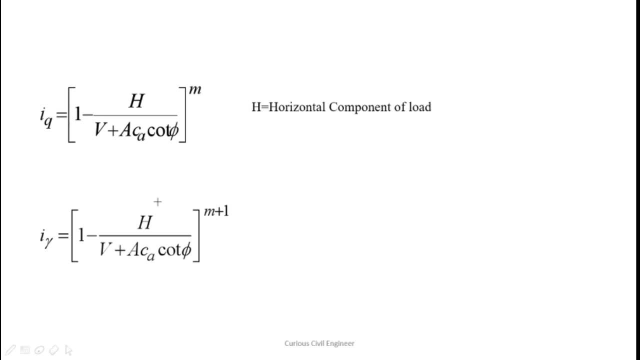 to remember this formula, ok. Next, The value of IQ is IQ and i gamma are given over here. where H is your horizontal component, V is the vertical component, A is the area of footing, CA is the adhesion value between footing and soil and phi is the angle of friction M. we have just seen, similarly, the formula. 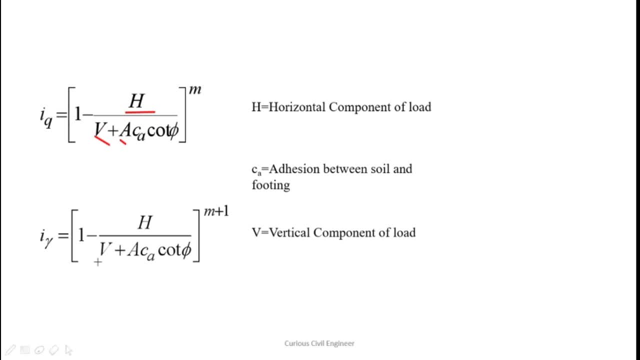 for i gamma is given over here, ok. and for say, for some reason, and if it is not given, this value of CA is, let's say this value of CA is not given into the numerical, what you will do. you will not just put the value as 1, don't worry about it if the area of footing is not. 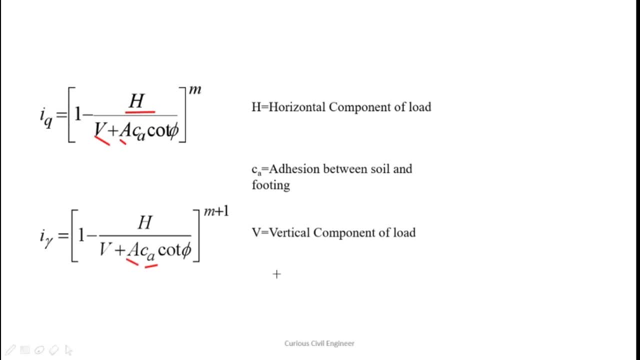 given. let's say, width is given 2 meter, length is not given. so what you will do? assume the length as a 1 meter. this area will be equals to L into B. that's it. it's very simple. the only thing is you have to remember lot of formulas. that's it, ok. this is so far about. 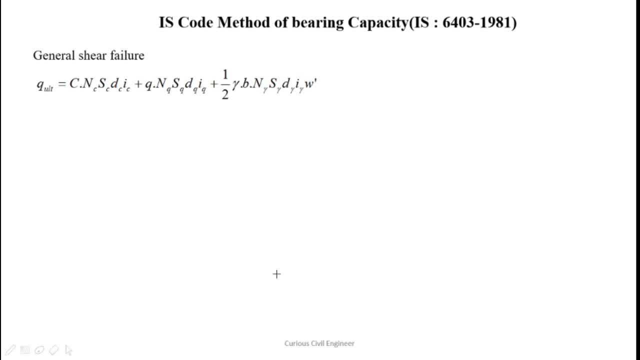 all the methods, The next very important method that is asked in examination so many time and probably it will be asked again this year or probably next year. this sorry, I am having little bit of cough for few days, so don't worry if you are wondering, it's not corona, probably I am. 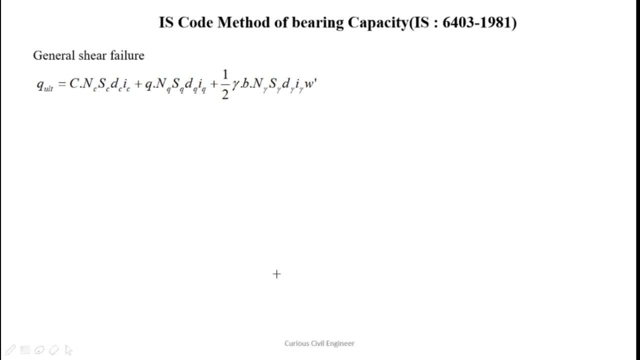 having cold. cold, let's say I am- let's hope I am having just cold. ok, so ice cold method that is given in IS6403.. Ok, This method is combination of all above methods that we have seen. ok, so it's little bit easier as compared with other methods. in some way it is little bit difficult. it totally depends. 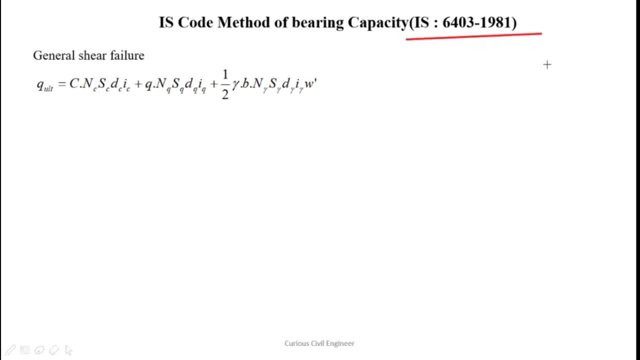 upon you. ok, so this is the formula and, if you could see the formula, the one new addition that you see over here, that is, the value of W dash. ok, W dash is given here. so in addition to shape factor, depth factor, inclination factor, we will also have to determine this W dash, which is nothing but water table factor. ok, we will. 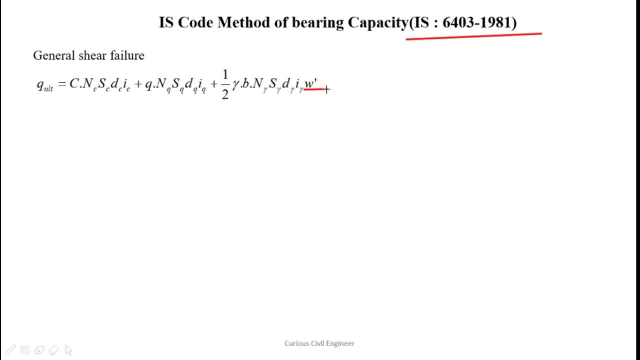 see how to do it. it's not very difficult. we already seen it into the effect of water table part, so if you have studied that, you won't find it very difficult. ok, let's go ahead. so, and in ice cold method, you have two different formulas. 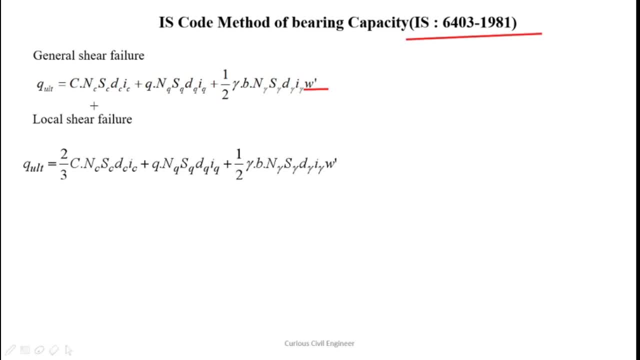 One formula for general share failure. other formula is for local share failure. so you need to pay a very close attention which type of failure type is given into your numerical if. if you have been given general share failure, make sure you are not using this formula. if you have been given local share failure, make sure you are using this formula. only it makes 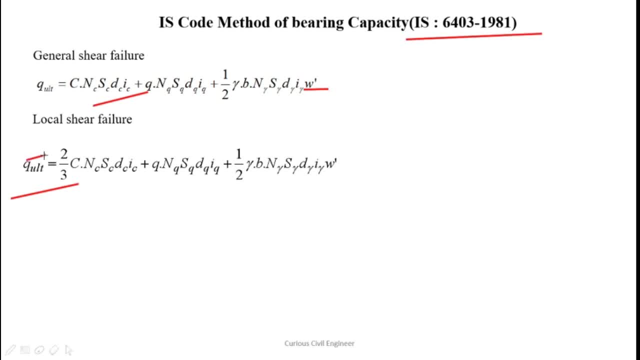 lot of difference. you should pay attention here. Ok, next one: NC, NQ, N gamma. as usual, they are same, but the only thing is the value of N gamma. hopefully, hopefully, the value of NC, NQ, N gamma will be given into your numerical. if they are not given, you have to remember these formulas. there is no other option available. 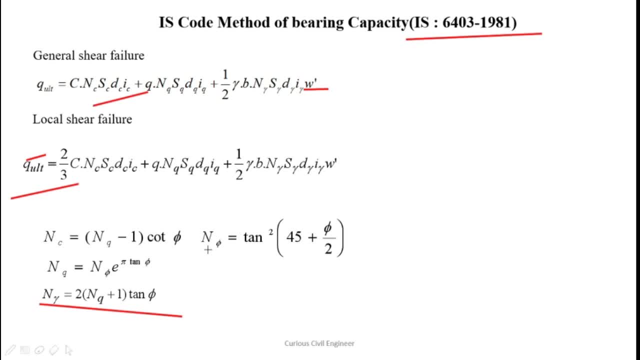 This formula for NC, NQ, N gamma. they are also given into the IS code, if IS codes are allowed in your examination. That is, go and use this table. go and use. there is a table on page number 8 and IS64031981. in this you can find out the value of NC, NQ, N, gamma. 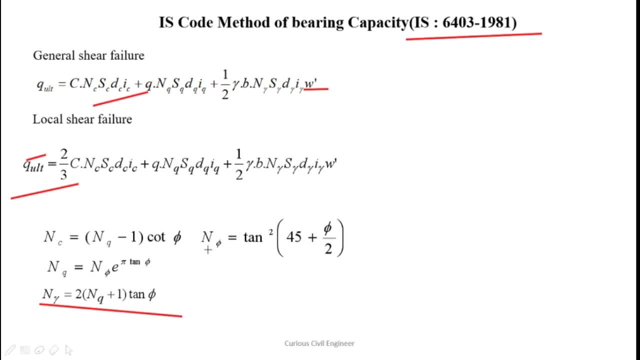 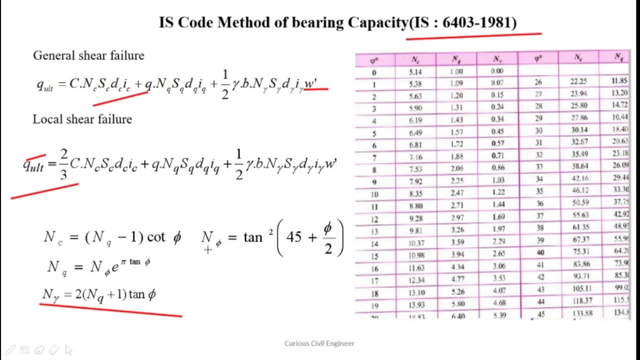 So I would say, to be on safe side, just remember this formula. ok, Next, this is also given. I have found this table. this table is given in, as I said, IS page number 8 of IS64031981.. Ok, To download this code, I will give you the link in the description. go and see for yourself. 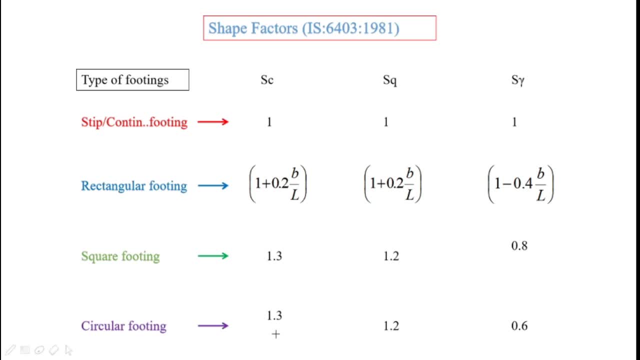 Next, these are the shape factor for IS code method. As I said, it is little bit easier than other methods because you don't have to remember the formula, you just have to remember the values. so for the strip footing, which is also called as continuous footing, 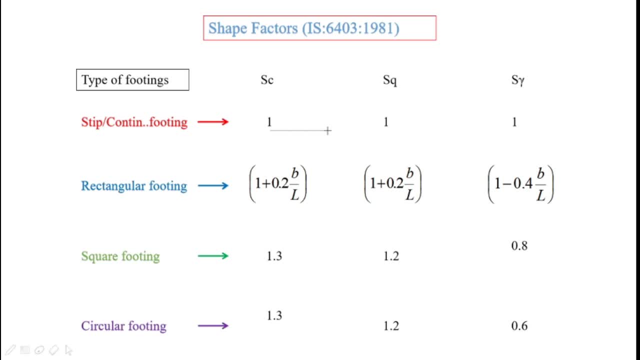 SUSQ and SGamma are 1, no need to worry about it. for rectangular footing: you have a formulas. these are the formula. remember it. square footing: these are the values. remember it. circular footing: you have different values. you need to remember all of these. if possible, take. 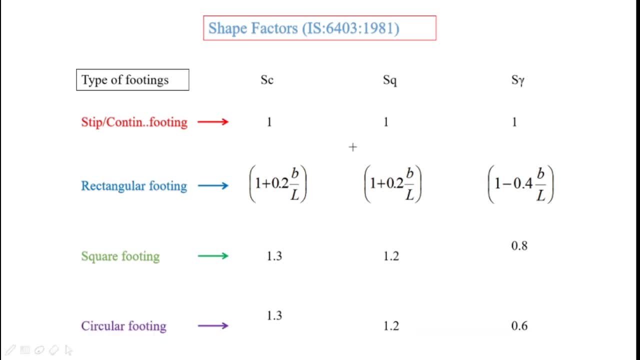 the screen shot, or I will do one thing: I will just upload this PPT into your Google Classroom, and so I will put this PPT into the description box where you can download it. Ok, Thank you very much. Ok, so remember this shape factor table. next one is a depth factor. depth factor: I will 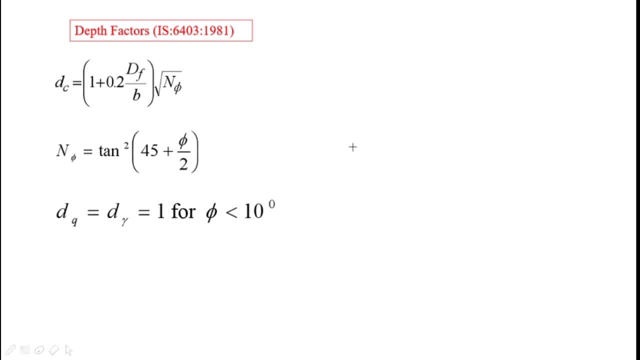 just give you the formula. I will not do much explanation because there is nothing much to explain beside that DC, DQ formula you have. this first formula is applicable when your phi is less than 10 degrees. if your phi is greater than 10 degrees, you have to use this. 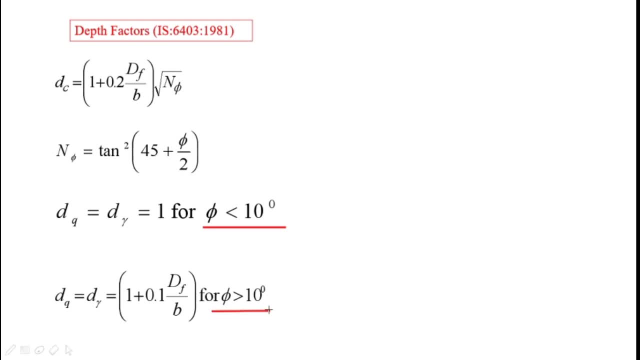 formula. So now some people might ask, what if the phi is greater than 10 degrees? So now some people might ask, what if the phi is greater than 10 degrees? you have to use this formula. If the phi is equal to 10 degrees, then it totally depends upon you use either of these. 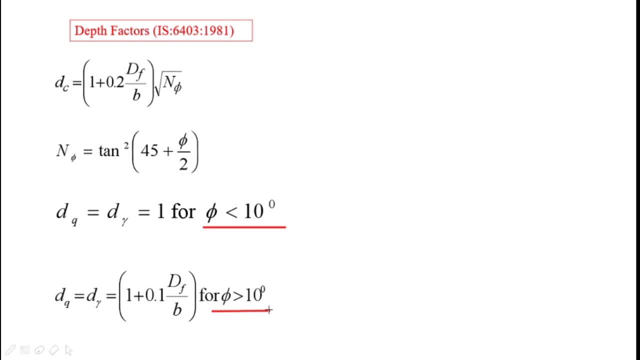 values. there is no issue at all. ok, depth factor is done and inclination factor. this is very important. I see an iq formulas here in front of you and, as we had discussed earlier, alpha is the angle between vertical and the load. ok, and anything else in this. 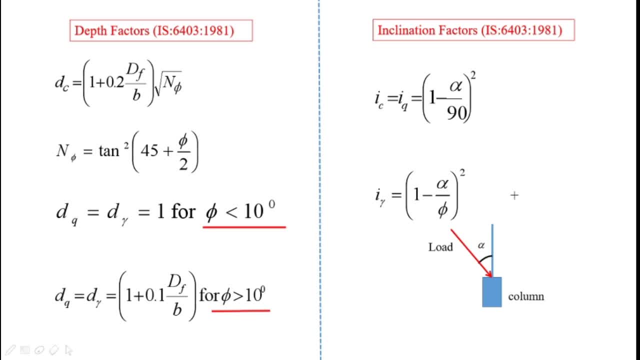 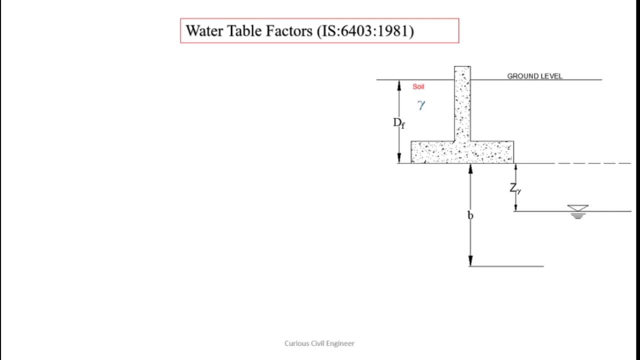 No, Ok, fine, let's go ahead. i'll not explain anything. it's very straightforward, okay, so this is the last bearing capacity factor that we have to see. so this is called as a water table factor. now you have seen that this is an additional factor that we need to consider in ice code method. so this: there are four different cases. 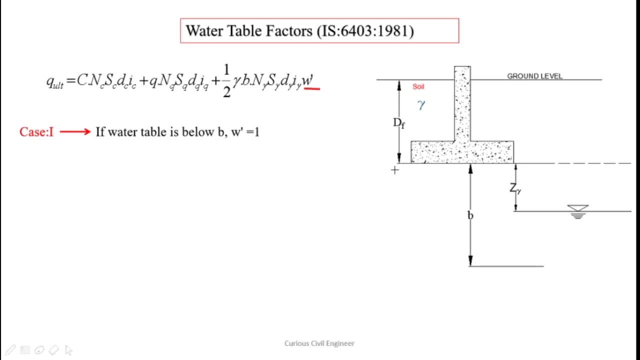 the case number one is when your water table is below the value b. so this is p, your width. and if your water table is below b, or exactly at b, okay, in these two, in these cases, the water table factor w dash equals to one. it means there is no effect of water table. this is we already seen in. 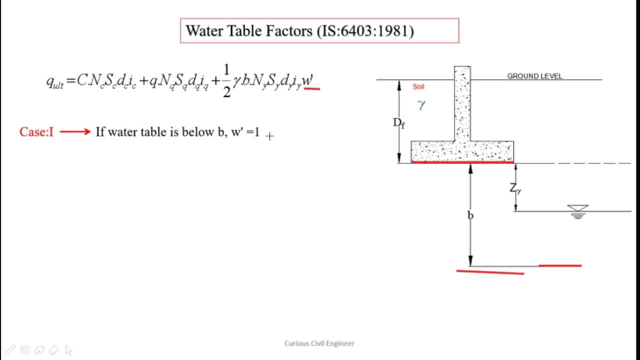 our video on effect of bearing capacity: effect of water table on bearing capacity. this is similar. case number two: when your water table is at depth tf. let's say your water table is at this position. let me rub it out. okay, let's say your water table is at this level. in this case, your w dash will be 0.5. 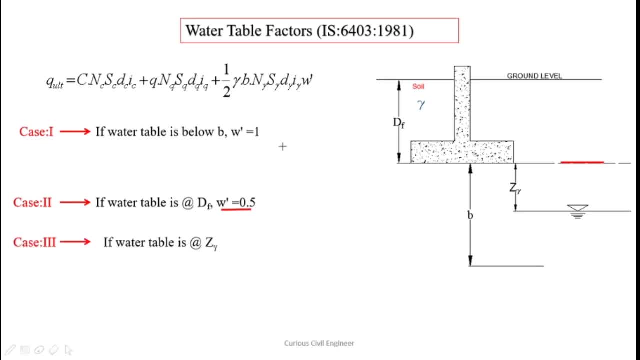 case number three: if your water table is at depth gamma z, so this gamma z is below the depth of, below the base of footing and above this distance p. in that case you have to use this formula: w dash equals to 0.5, 1 plus gamma, z, gamma by b. what is z, gamma, z, gamma? remember? 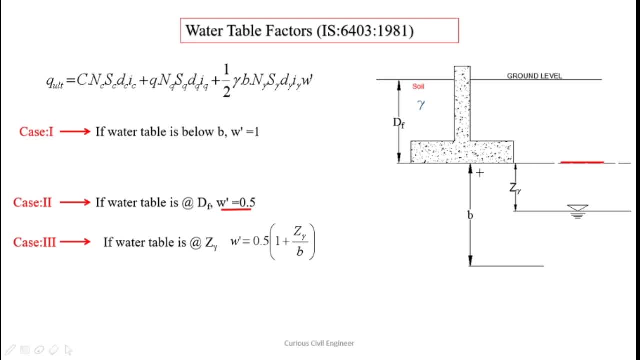 z, gamma is always below the base of footing but above the distance p. now the case 4. case 4 is little bit complicated, so let's look at the case 4. now the case 4 is a little bit complicated. if the water table is above the base of footing but below the ground level, that means if the water 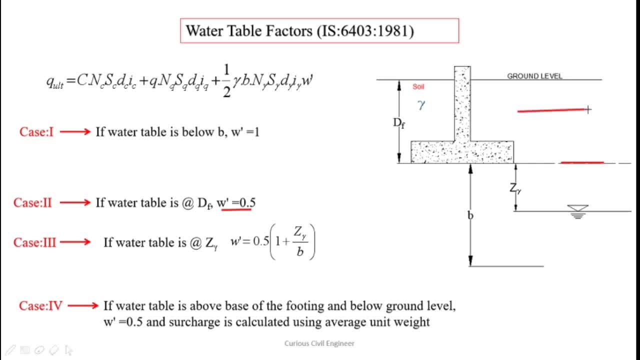 table is, let's say, over here. in that case the w dash will be 0.5, but the surcharge is calculated using average unit weight. now what is the surcharge? this is the value of surcharge. how do we calculate surcharge? surcharge is nothing, but q equals to this. q equals to 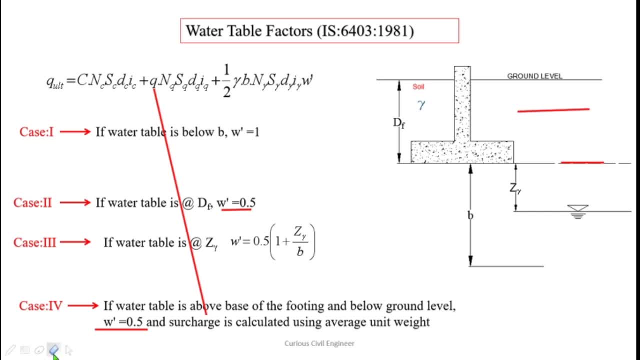 gamma into df. okay, so when you are calculating q equals to gamma into df, the unit weight, that is, the gamma, should be gamma average. how do we take the average? let's say your water table is somewhere over here. okay, that means this unit weight above the water table will. 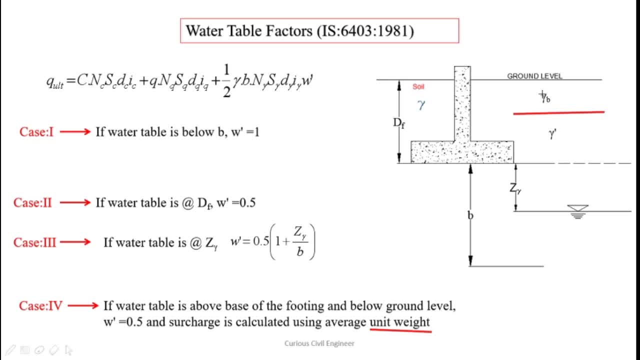 be gamma bulk and the unit weight of water below the water table unit weight of water is going to be 100 местups. okay for enührung, and enter means this Nahaling is always going to be рав cut. so weight of soil below the water table will be gamma submerged. so let's say this df is 5 meters.